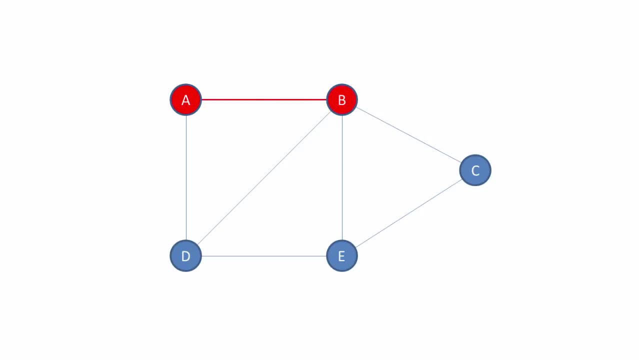 In the case of our simple graph, we simply follow a path of vertices until we've exhausted all of the vertices in the graph. It's easier to see how this works with a more complex graph, Starting with vertex first traversal. We follow a path until we can go no further. 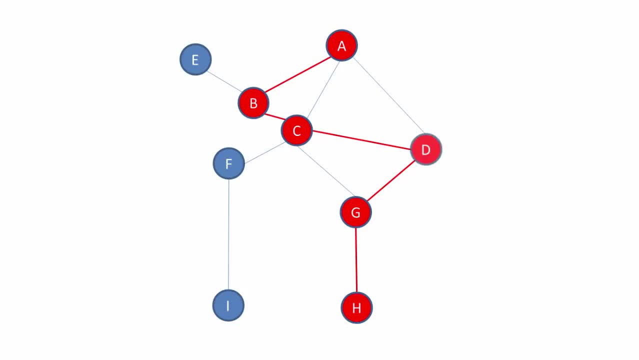 Now we backtrack and as we do so we ask if there are any more paths to explore. Here we can see there's another path which we will explore until it's exhausted, And then we backtrack again until such time as we find another path to explore. 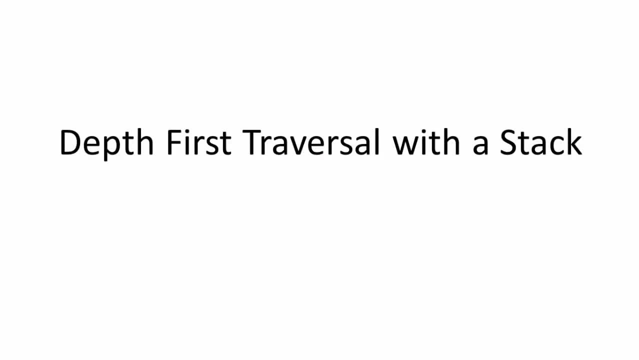 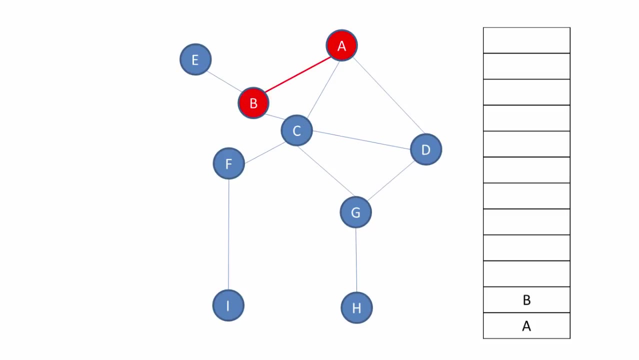 So how is this done programmatically? Depth first traversal. Depth first traversal can be managed by means of a stack data structure. Here's our graph and here's a stack. As we follow a path of vertices, we push each vertex onto the stack until such time as the path is exhausted. 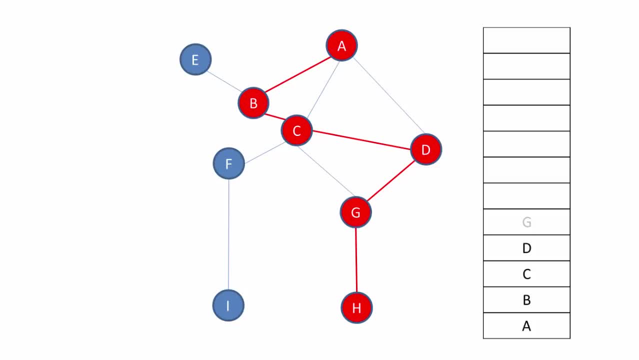 Backtracking involves popping vertices off the stack, one at a time, until such time as we come across a vertex which has adjacent unvisited vertices, in this case vertex C. So then we explore this path, pushing vertices onto the stack as we go. Once that path is exhausted, we again start popping vertices from the stack. 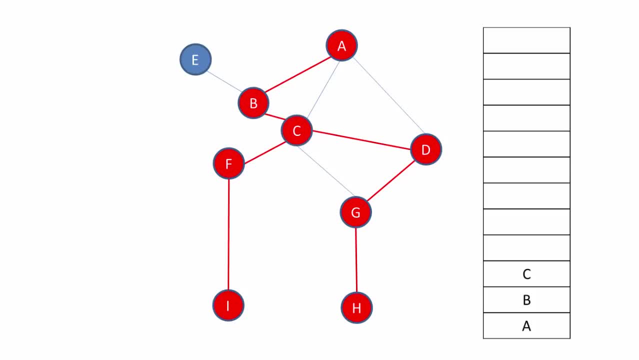 until such time as we find one with unvisited adjacent vertices- in this case B, We have another path to explore. Once that path is exhausted, again we start popping vertices from the stack. Eventually, we'll reach a situation where the stack is empty. 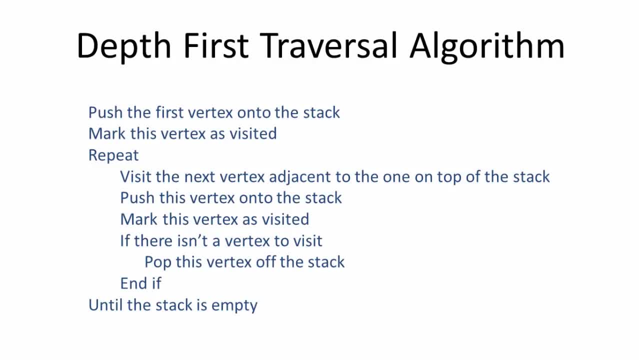 Here's an algorithm for depth: first traversal of a graph, As you've seen. then we push the first vertex onto the stack and mark it as visited. Then we repeatedly visit the next vertex, The next vertex adjacent to the one at the top of the stack. 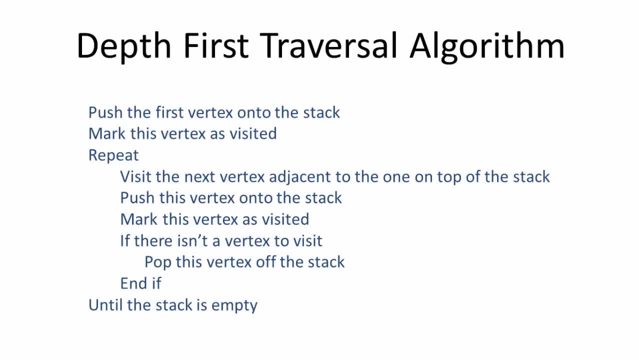 We push anything we come across onto the top of the stack, mark it as visited, and we do this until there isn't anything else left to push onto the stack. So then we pop another one off the stack. We keep doing this until such time as the stack is empty. 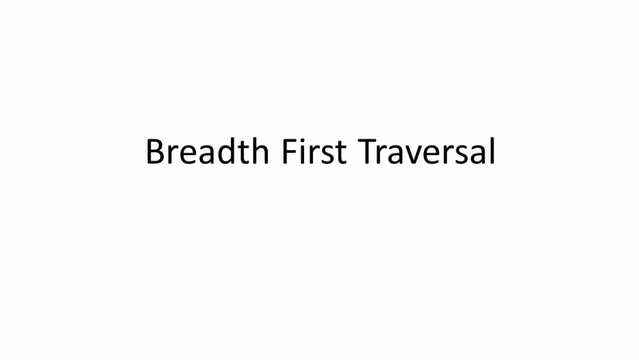 So how does breadth first traversal work? Breadth first traversal starts at the first vertex and tries to visit all of the vertices as close to this vertex as possible. We're effectively moving through the graph layer by layer, first examining the layers closer to the first vertex. 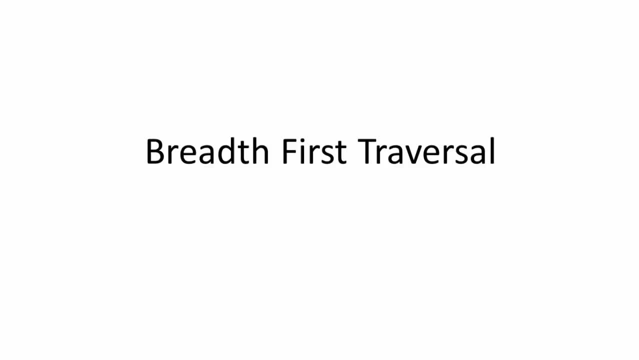 and then moving down to the layers furthest away from the starting vertex. Let's see that with our simple graph We examine everything close to A and then we examine everything close to B. Let's see that with a more complex graph You can see in this case we're definitely moving down through the layers. 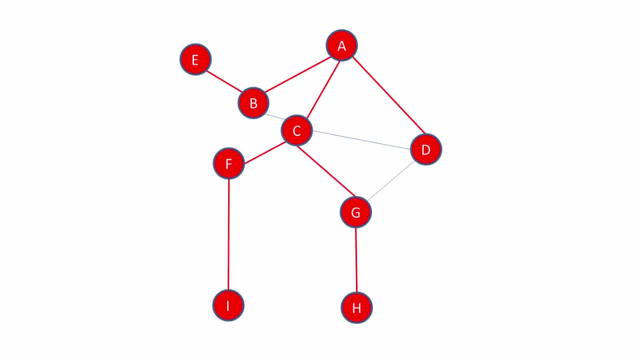 until such time as we've traversed the entire graph Breadth. first traversal can be managed using a queue data structure. We visit the first vertex and then we visit all of the adjacent vertices, in queuing each one as we go, Once we've visited all of the unvisited vertices, 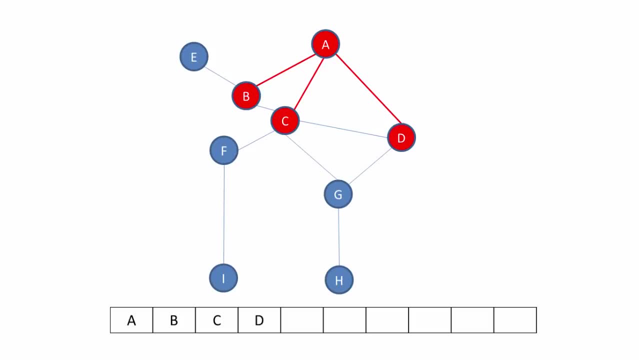 adjacent to the first vertex. we dequeue the first vertex And then we examine the one at the front of the queue to see if there are any more unvisited adjacent vertices. In this case, B has one, So we visit E and we enqueue it. 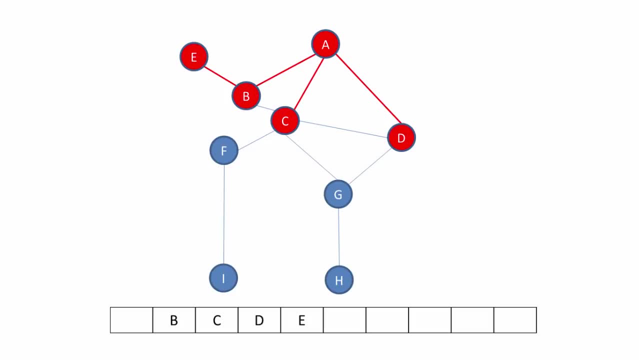 Now that there are no more unvisited vertices adjacent to B, we dequeue B And now C is the current vertex, And here we find F and we find G, which again are visited and added to the queue. Now that we've exhausted all of the adjacent vertices, next to C 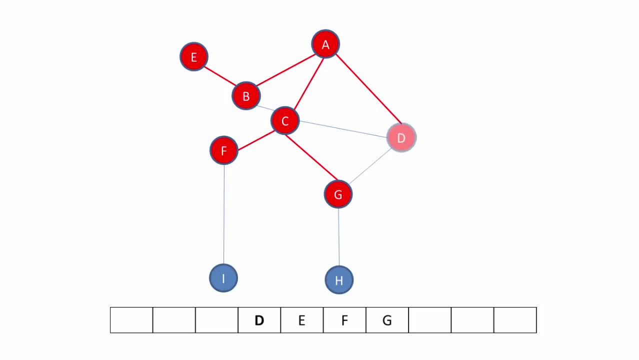 we dequeue C. D is now at the front of the queue, but D has no adjacent unvisited vertices, so we dequeue D. E is now at the front of the queue and it has no adjacent unvisited vertices, so we dequeue E. F is at the front of the queue.